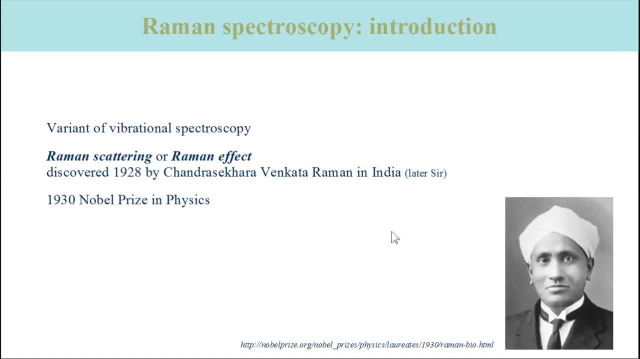 of the bright sunlight in India. Very soon afterwards he received the Nobel Prize in Physics for his discovery. He was also knighted in 1929 by the Queen of England and became Sir Raman. In Raman, spectroscopy light that is inelastically. 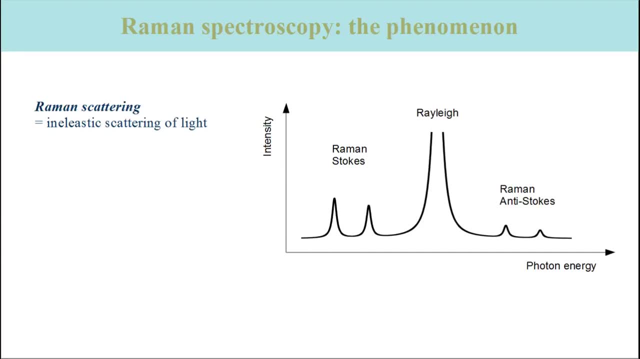 scattered is detected. Inelastic scattering means that the scattered photons have a different energy Then the incident photons. This scattering is called Raman scattering. The figure shows a hypothetical spectrum of Rayleigh and Raman scattering from a simple compound. Most of the light that is scattered is elastically scattered, which means that the scattered 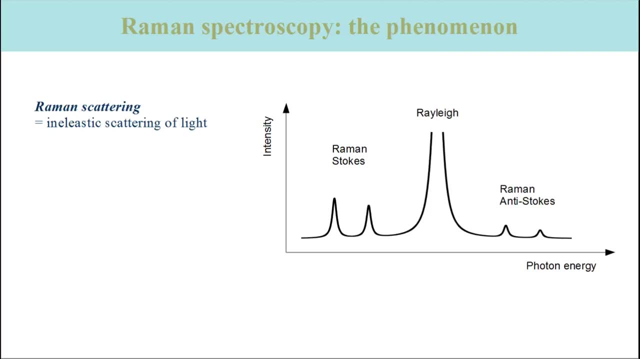 photons have the same energy as the incident photons. This is Rayleigh scattering. However, some of the photons have less energy And some have more energy than the incident photons. This is Raman scattering, which gives rise to additional lines in the spectrum of scattered radiation. If lines are found at 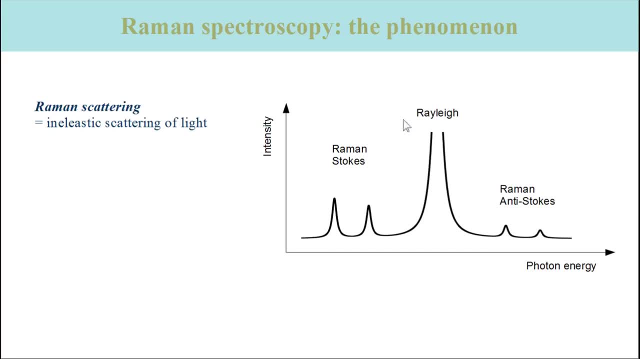 smaller energy than the Rayleigh line, they are called Stokes lines. If they have more energy, they are called anti-Stokes lines. It turns out that the energy difference between the Rayleigh photons and the Raman photons corresponds to the energy needed for. 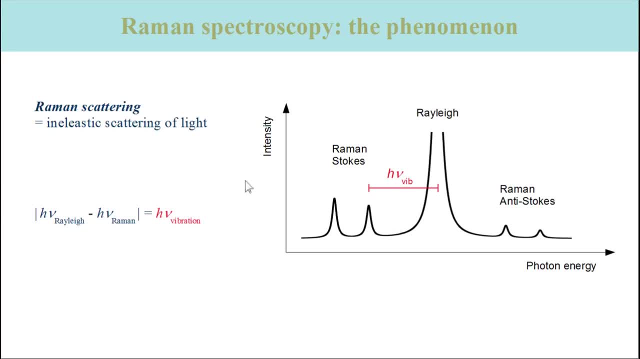 vibrational transitions of the scattered molecule, Scattering is a rather unlikely process. The probability for Rayleigh scattering is ten to the power of minus four, meaning that only one out of ten to the power of four photons is rarely scattered. Raman scattering is even less likely. the probability is about 10 to the power of minus 9.. 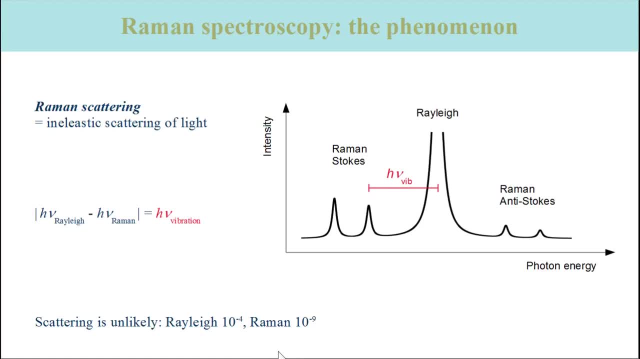 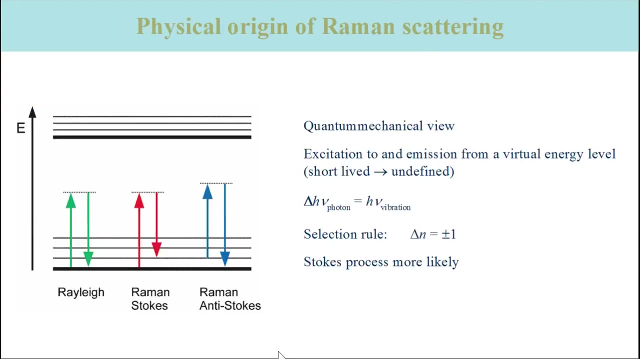 This is a disadvantage of Raman spectroscopy, because only a very small fraction of the incident photons generate a Raman signal which limits the signal-to-noise ratio. What is the origin of the Raman bands in the spectrum of the scattered photons? 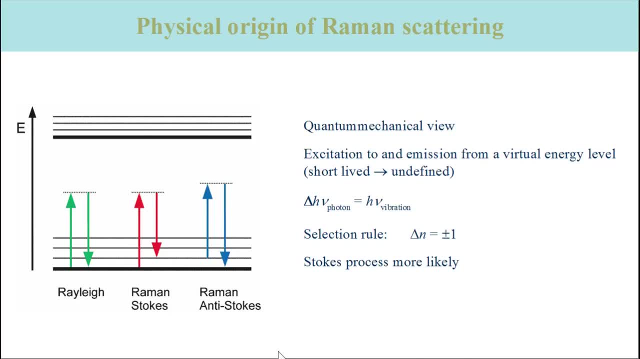 This is easy to understand in the quantum mechanical view, which is illustrated in this figure. The figure shows the vibronic states of a molecule for the electronic ground state here and for the first electronically excited state, as well as three processes as well as two processes. 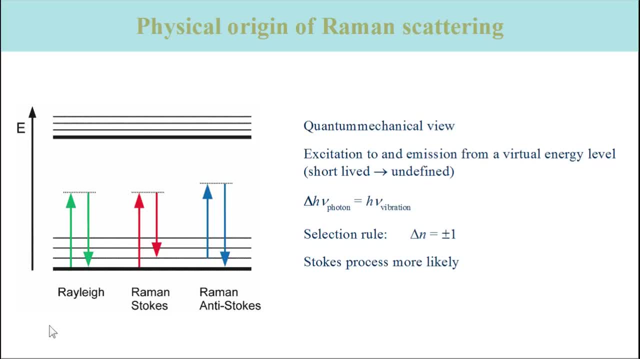 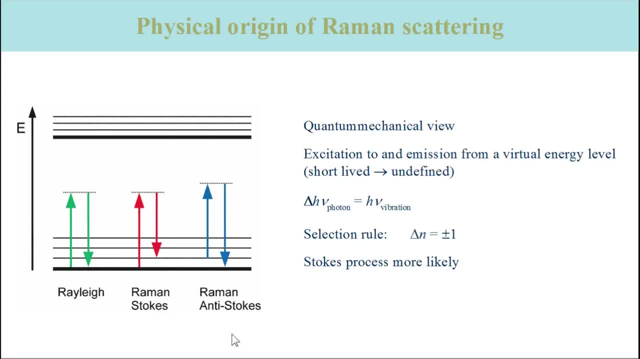 that the photon energy is less than required to excite the molecule to a higher electronic level. In all of these processes an incident photon interacts with the molecule and excites it to a virtual state. The photon becomes annihilated in this process. The virtual state is a non-stationary state of the system. 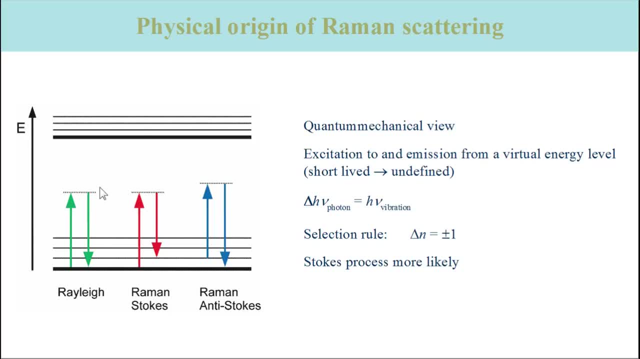 It has therefore a very short lifetime and its energy is not well defined. When it decays, the scattered photon is created. The three processes differ in the energy of the scattered photon. In Rayleigh scattering, indicated by the green arrows, the photon energy of the scattered photon is the same as that of the incident photon. 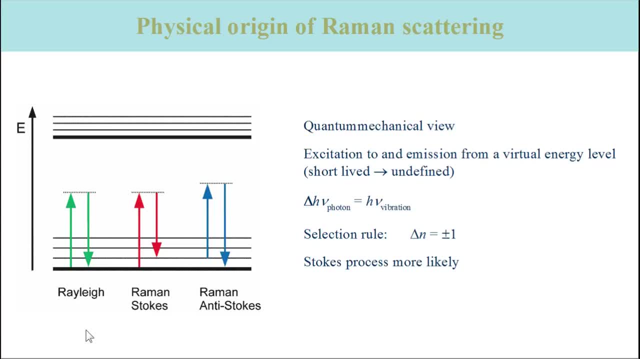 Therefore, there is no net energy transfer between radiation and the molecule And the final state of the molecule is the same as the initial state In Stokes-Raman: scattering. the energy of the scattered photon is less than that of the incident photon. Understand these differences. 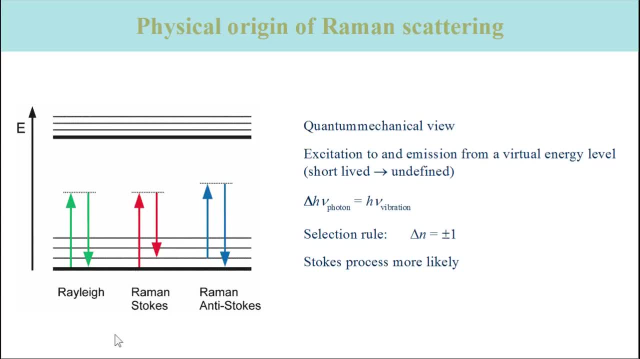 Listen carefully, please. The energy difference is used to excite the molecule to a higher vibrational state. Only transitions to the next vibrational level are allowed in Raman spectroscopy. This is the same selection rule that applies for the absorption of infrared radiation. 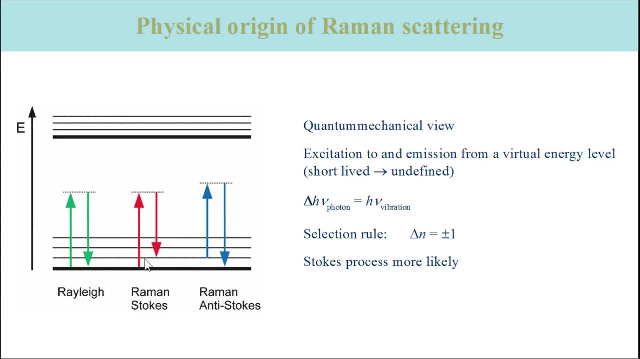 Therefore, the difference in energy between the incident photon and the scattered photon matches that of a vibrational transition: h, nu, vib. As most of the oscillators are in the vibrational ground state at room temperature, the most relevant process for Stokes Raman scattering is from the vibrational ground state to the first excited vibrational state.